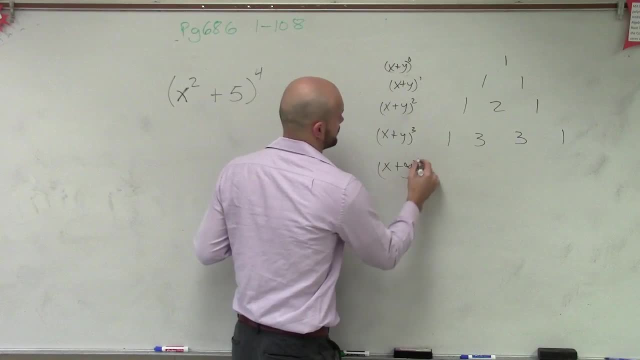 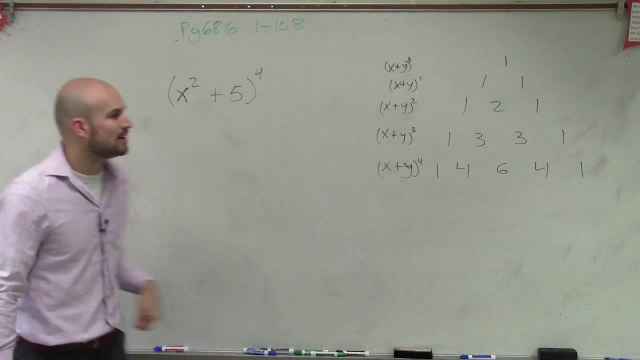 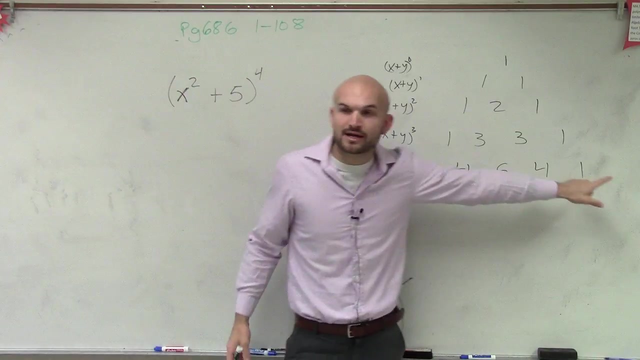 then if I expand a binomial to the fourth power, my coefficients are gonna be multiplied by 1, 4, 6, 4, 1.. So that's by using Pascal's triangle to say: all right, each one of my coefficients. if I just had x plus y, these would be my. 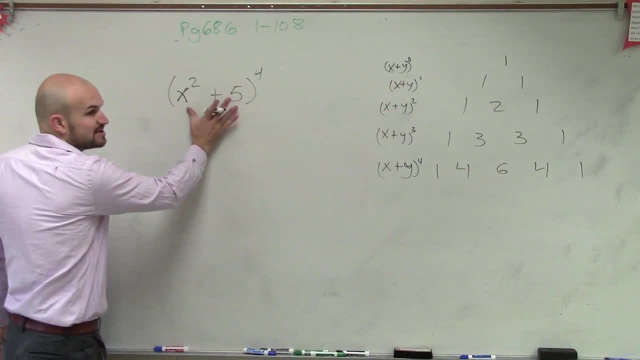 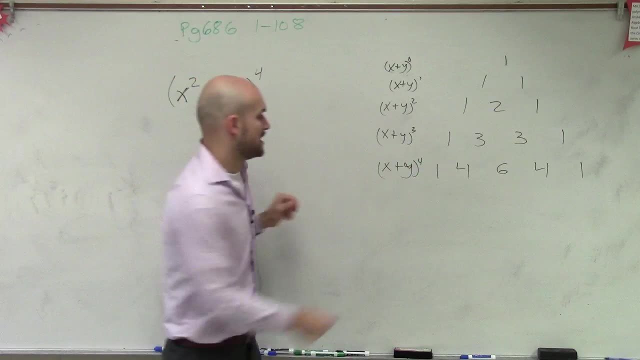 coefficients. However, we look at this and we have some different terms here, also with different degrees, And the next thing we also learned is remember that we start at your degree. this was your n right And every term can be written as x to the. 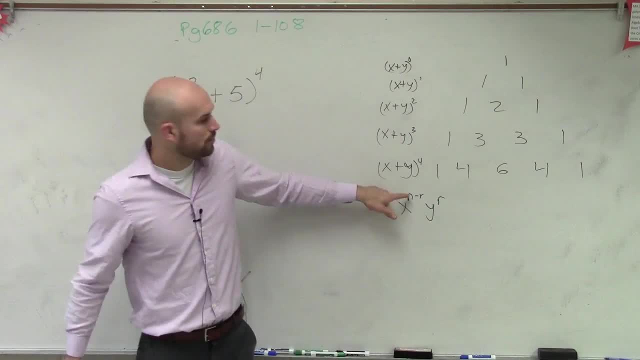 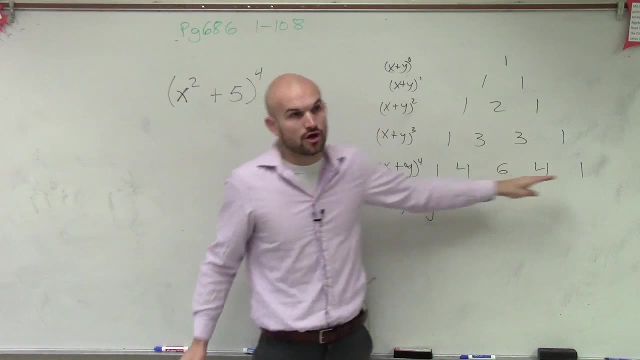 n minus r times y to the r where your degree of your first term goes down. in descending order, It starts at n, where r is 0, and then goes all the way down to 0. And your r starts at 0 and then ascends all the way up to your higher. 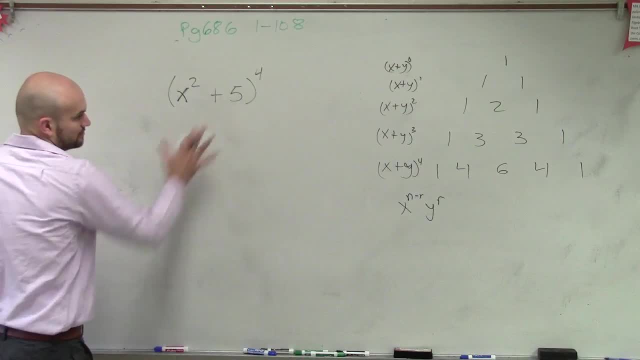 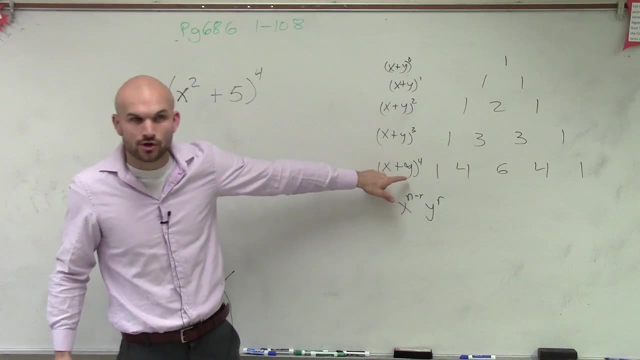 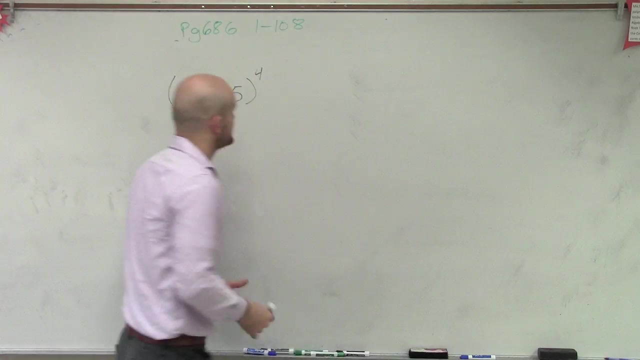 degree. So when I'm trying to figure this out, I know that binomial expansion to the fourth degree. I'm gonna start with every single term being multiplied by these coefficients. So I have 1, 4, 6, 4, 1.. So what I'm going to do is to get this started. I'm just gonna 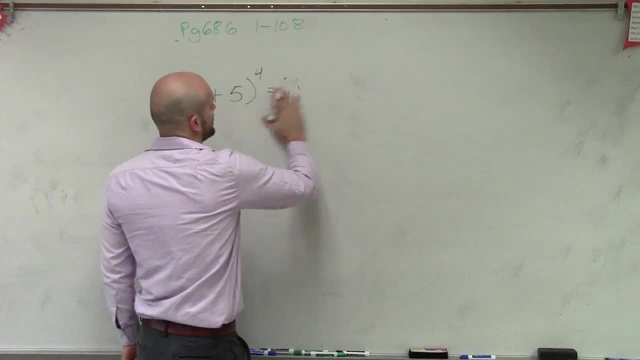 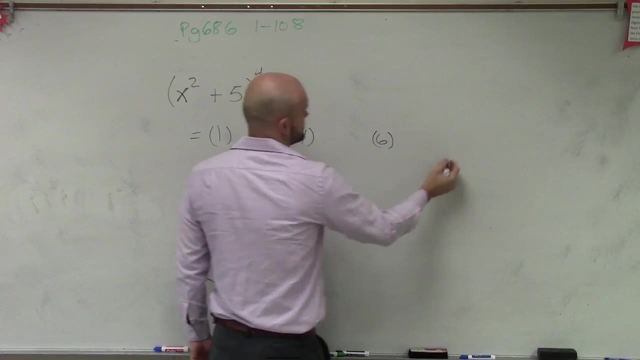 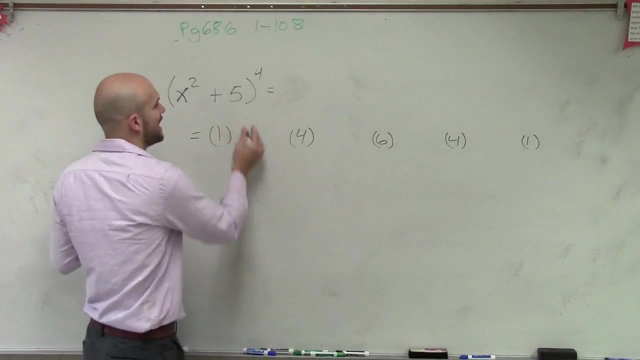 write 1.. I know that my first term's gonna be multiplied. ah, let's write it down here: First term's gonna be multiplied by 1, then multiplied by 4, multiplied by 6, multiplied by 4,, multiplied by 1.. Alright, And then what we know is we could have every single. 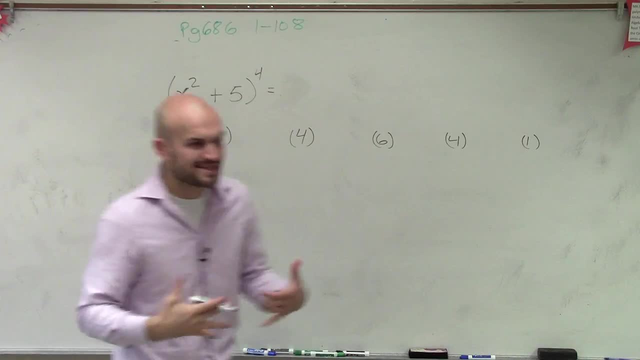 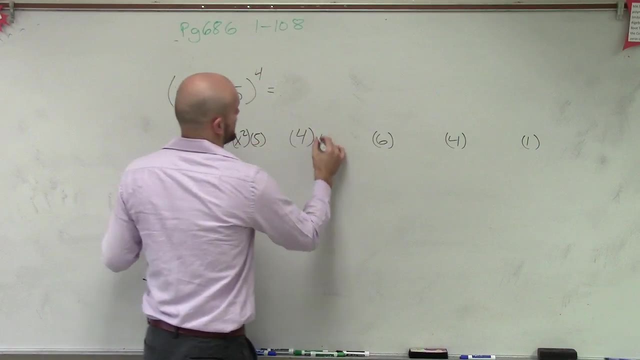 one of these is gonna be a term. ah, what I'll do is I'll rewrite every single term in there. So let's write x squared- 5. x squared. you don't have to do all this work, but I'm. 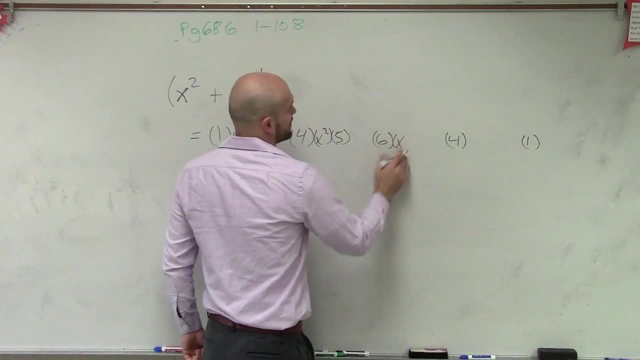 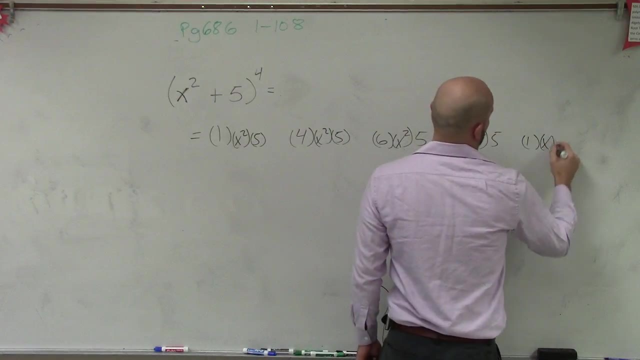 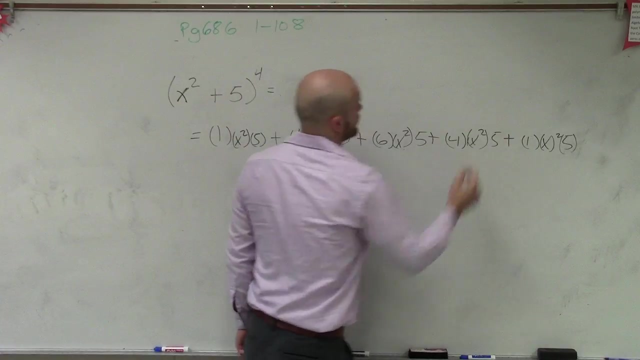 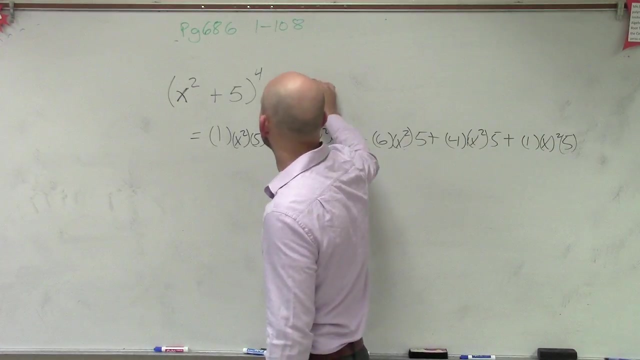 just gonna kinda show you, where you guys can, what it looks like, so then we can start doing some shortcuts. Okay, So here, ladies and gentlemen, we're gonna have every single term of our binomial expansion. But remember, a binomial expansion can always be written as x to the n minus. 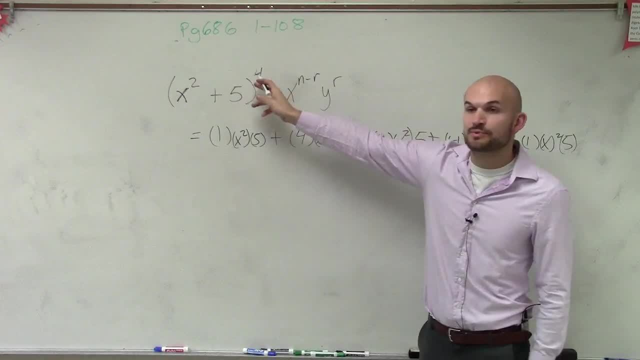 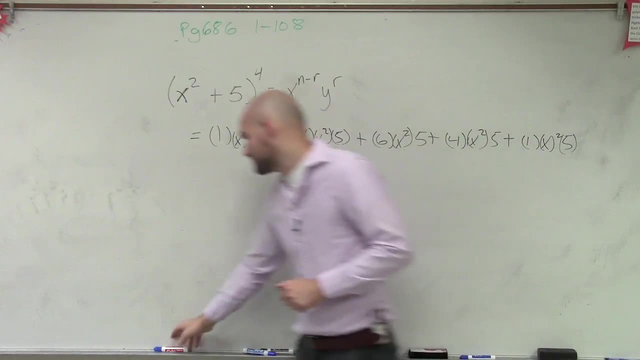 r times, y to the r. So what we're gonna do is we're gonna start with our 4, um, with 4 as being our n, and r being 0. So what we could have is say this is going to be to the. 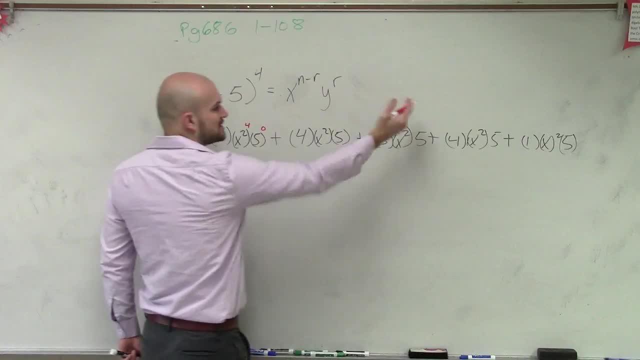 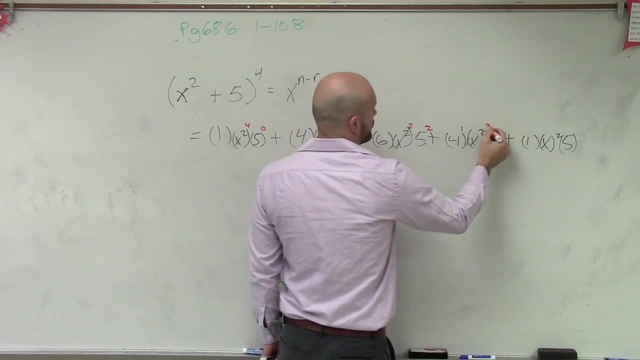 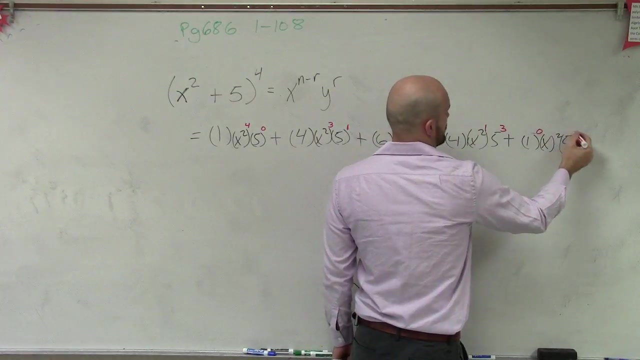 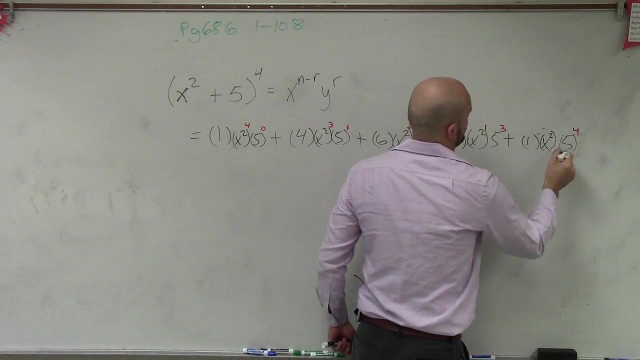 fourth To 0.. And then, remember, the first term now goes in descending order, So that's 3, 1, 2, 2, 1, 3, 0, sorry, Okay. So do you guys see how, what this is doing? 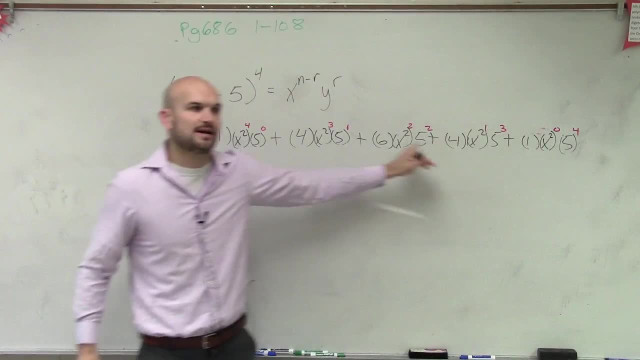 Okay, So do you guys see how what this is doing? Okay, So do you guys see how what this is doing? Okay, uh, you guys didn't see it, but it's酷 Right. First of all, you notice some of my coefficients. My coefficients I obtained from my 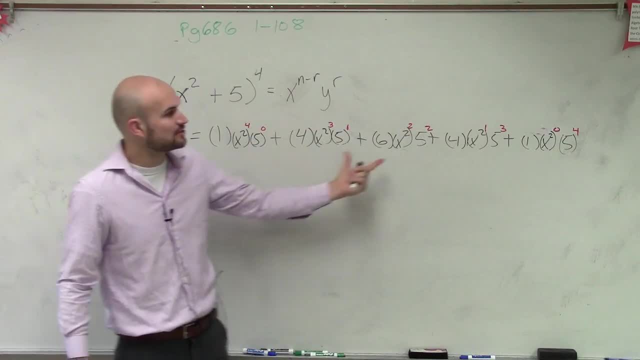 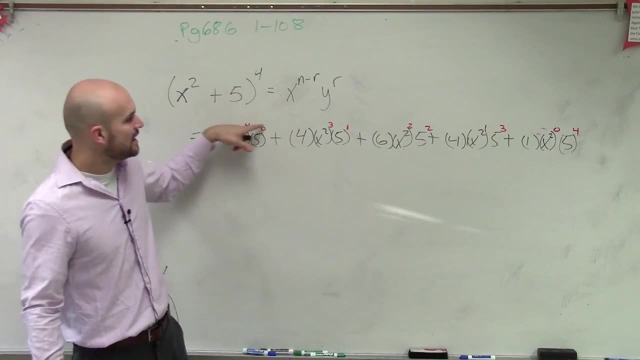 Paschall's Triangle. In the binomial expansion we have every single term. but notice how the R, notice how the relationship between the exponents: For the first term it starts at your degree and then goes down. See how x, squared, first starts at 4, then goes to. 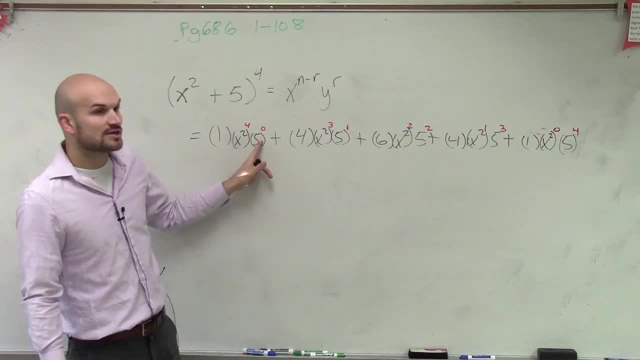 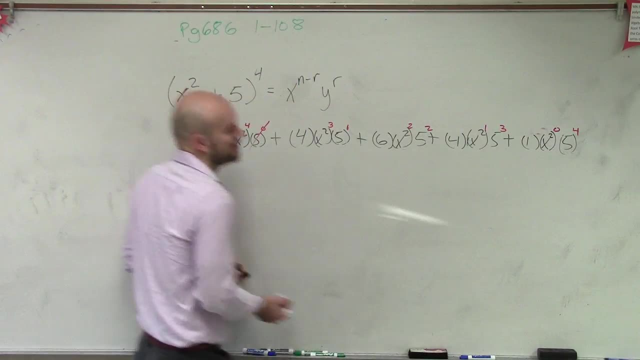 3,, 2,, 1, and then 0? Right. And then your second term starts at 0 and then climbs all the way up to 4, or ascends up to 4.. Now we don't need to write these, but I just wrote. 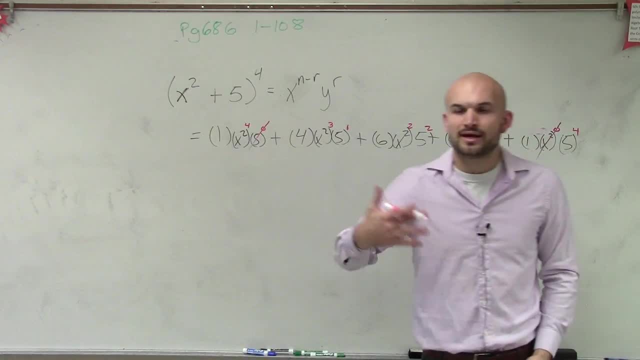 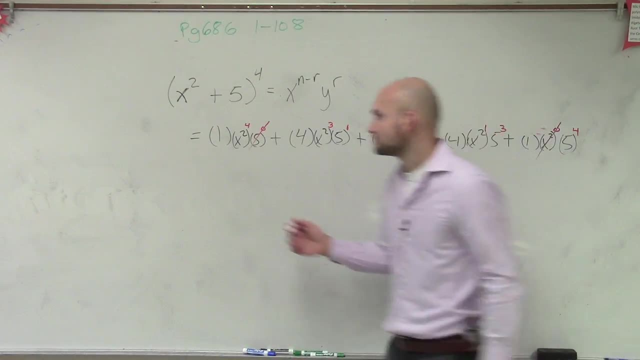 them in there, because that's a whole other problem. Okay, we know those go to 1, but I just wanted to show you it occurs with every single one of these terms. So now what we need to do is just simply simplify our process, So remember. 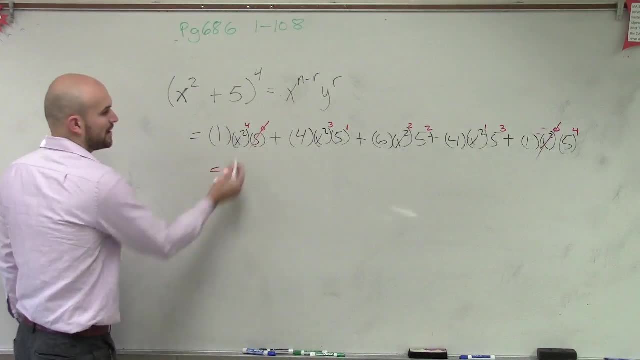 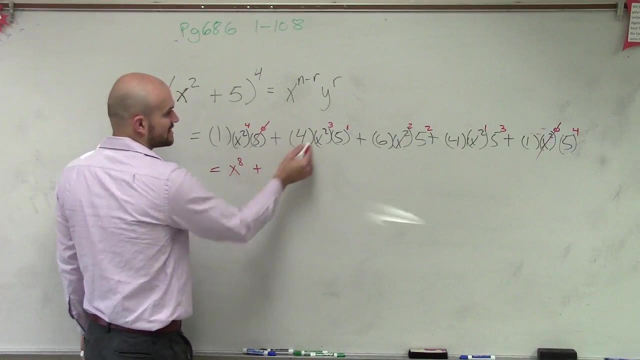 when you take an exponent and raise it to a power that's going to leave you multiply. so x squared to the 4th is x to the 8th, plus x squared cubed is going to be x to the 6th. 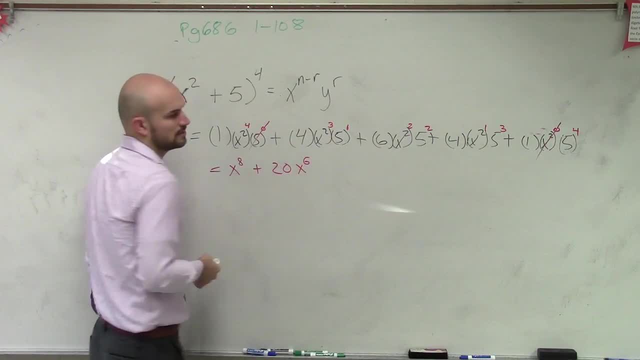 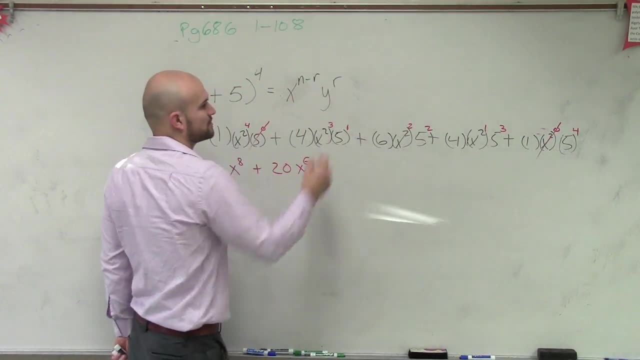 and 4 times 5 is 20, so we can just multiply those plus 5 squared is 25, times 6 is 150, x squared, x squared or x squared squared is going to be x to the 4th, so we have 150. 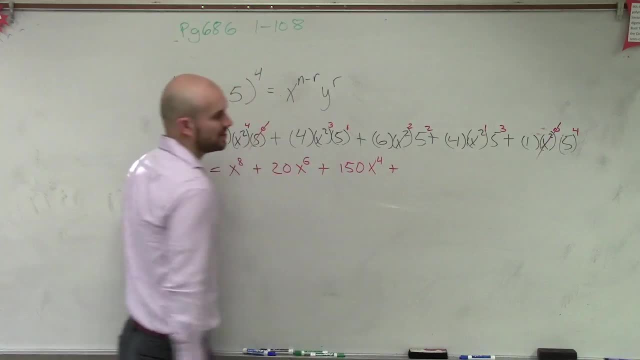 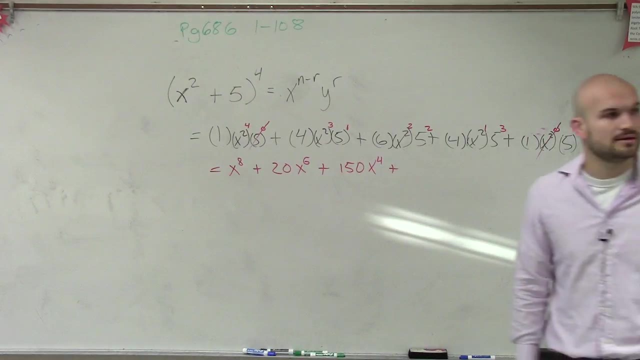 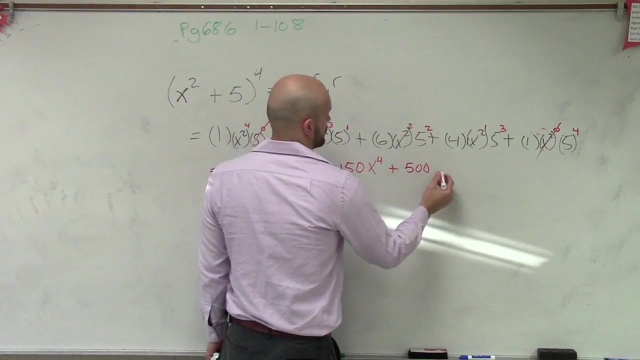 x to the 4th plus 5, cubed is going to be 125, times 4 is going to be, let's see, 400, so then times 4 would be 500.. Now what I'm doing is just simplifying each term and then 5 to the 4th.